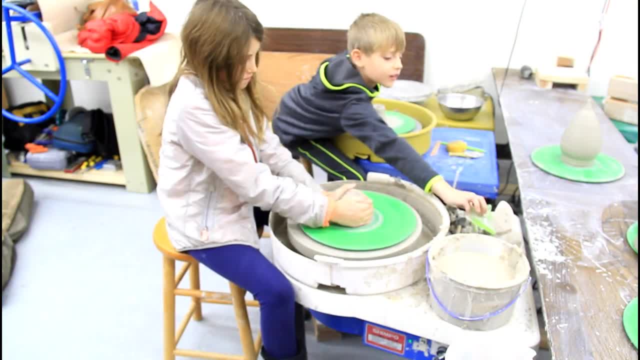 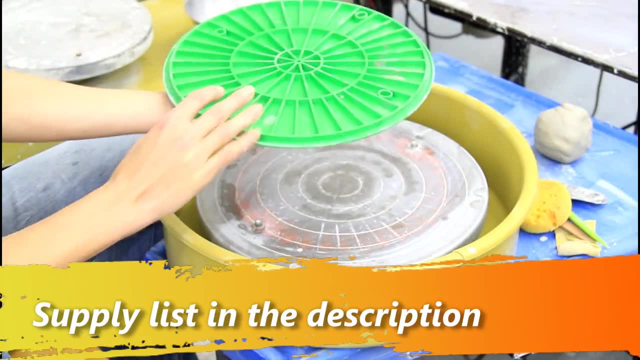 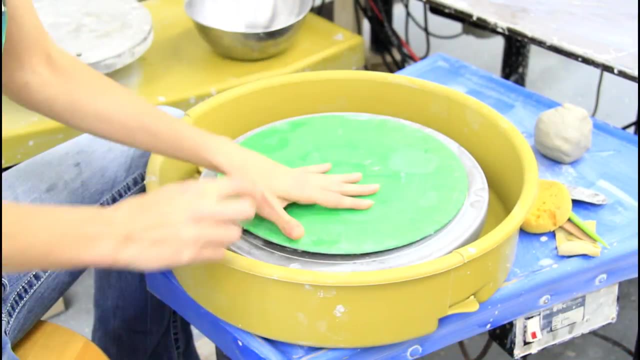 make pottery on a pottery wheel. Thanks to Valley Pottery for letting us use their pottery wheels. This is a pottery wheel, and to set up a pottery wheel you want to have a bat. See the holes right here. You just set it on top of your pottery wheel. You have your foot pedal. This will control. 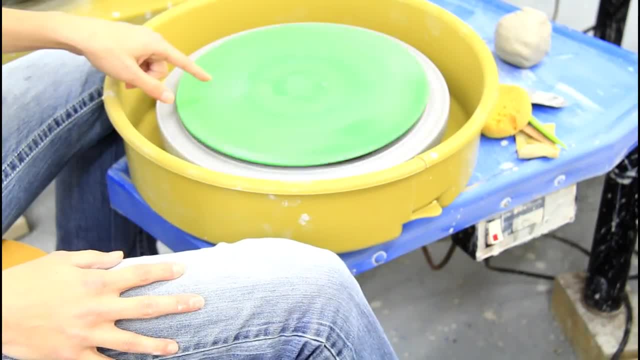 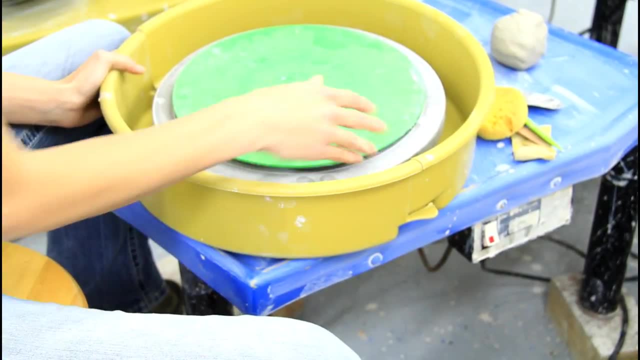 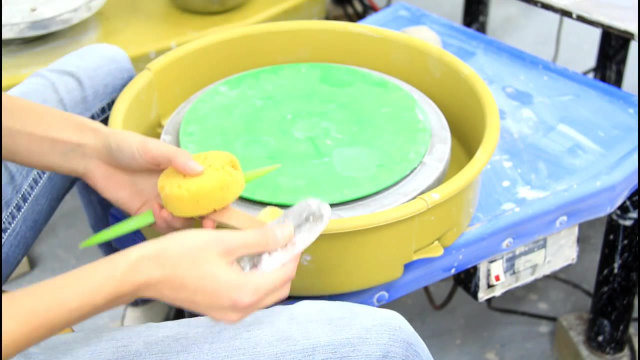 how fast your wheel moves. Okay, so you have to get used to how fast you're pushing and get control that way. This is a splash guard. This is going to keep all the splashing of this clay off of you- Not all of it, but some of it. You want to grab some tools. You want a bucket of water. 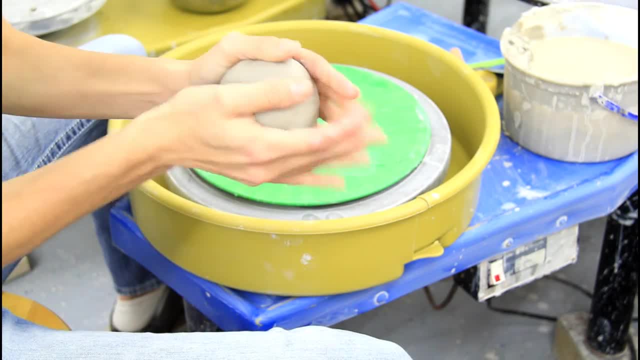 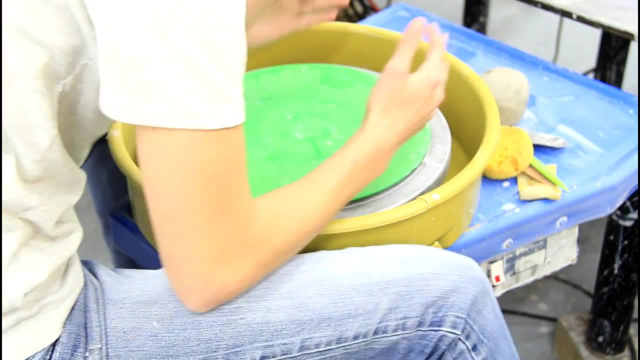 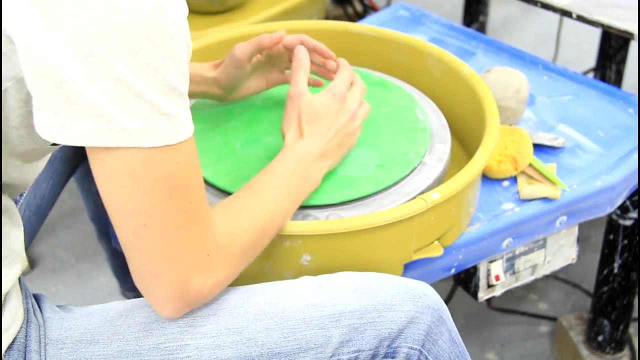 You want to grab a piece of clay and form it into a ball, like this, and use it down. You want to straddle the pottery wheel like this, and then- I like to get comfortable with this- Push it back, Push it forward, and then you want to rest your elbows on your legs, like this. Okay, so you're. 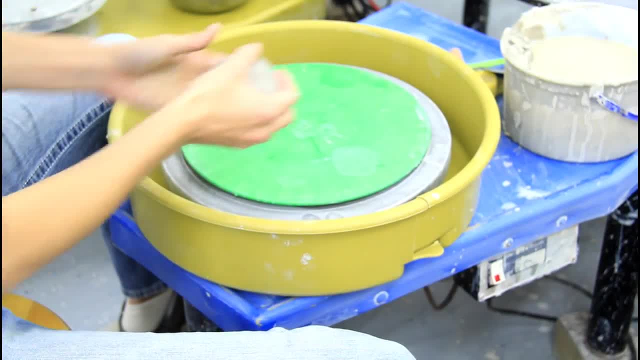 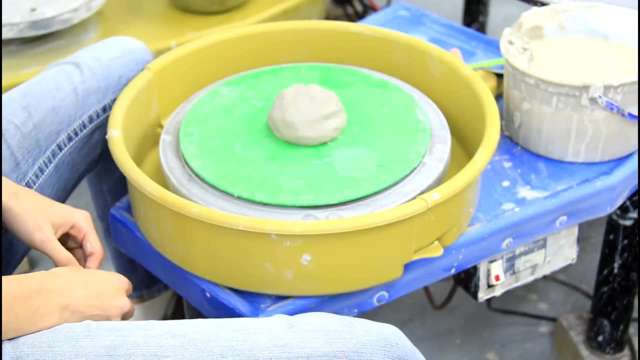 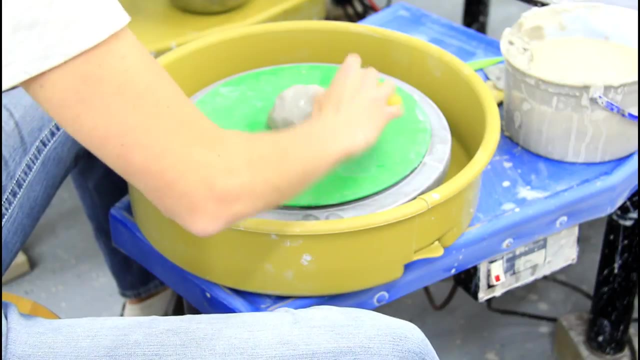 going to take your clay, Your circle clay, and you're going to slam it right in the middle of your bat. So you just take your arm, go flat like that. Okay, be aggressive. Then you want to grab your sponge and add some water to your circle right here. I like to add it to my hands too. Get in a good position and then I start. 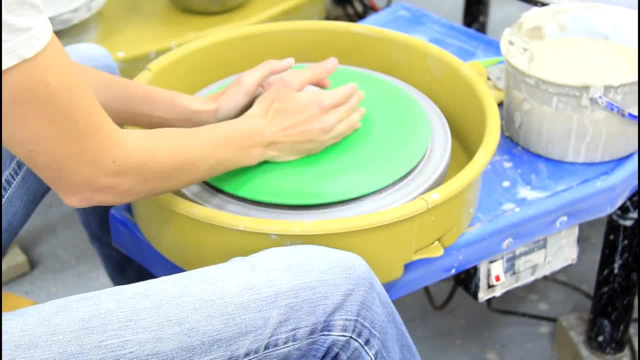 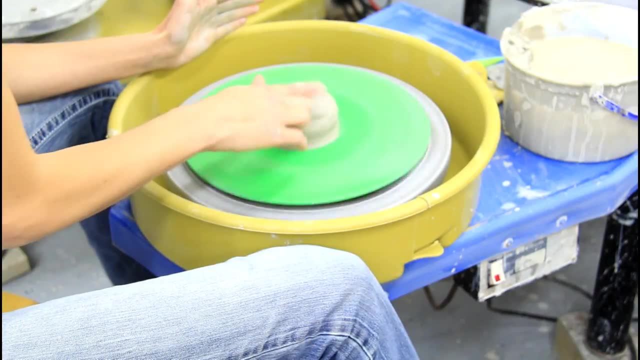 right on those my hands. Now what I'm going to do right now is I'm going to make sure that it's centered, so I'm kind of pushing A little bit. see how it's wobbly like that. That means it's not centered and you want to keep your. 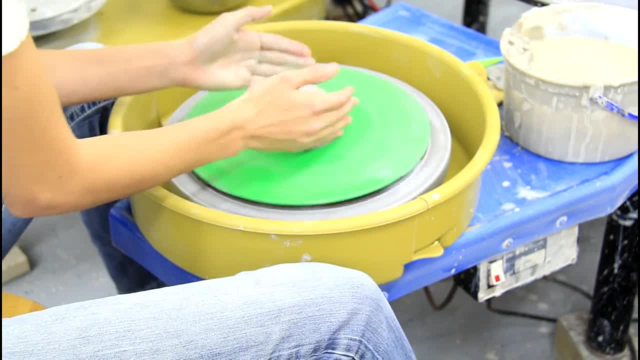 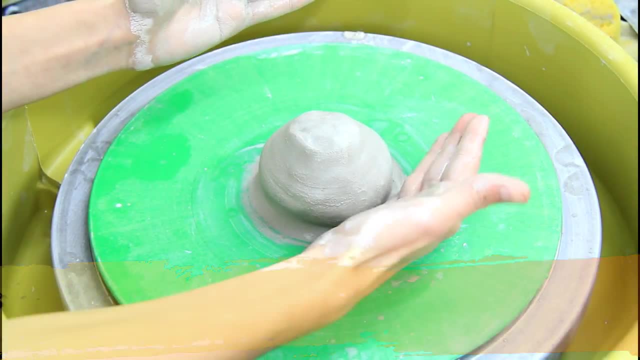 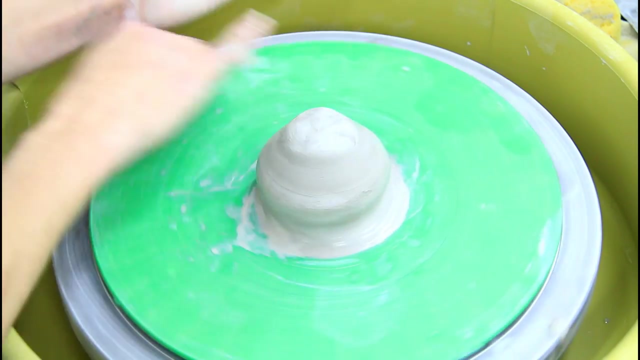 hands wet, because if they get sticky then it'll really pull your clay around. Okay, so what we're going to do is we're going to make what's called a cone and I'm going to push with this hand and then pull up with this hand. So this one's going to push and this one make sure that I don't push. 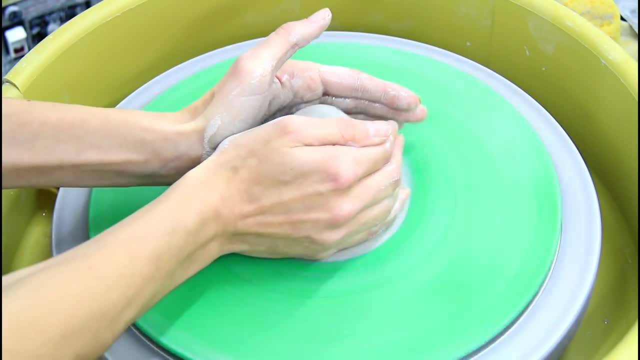 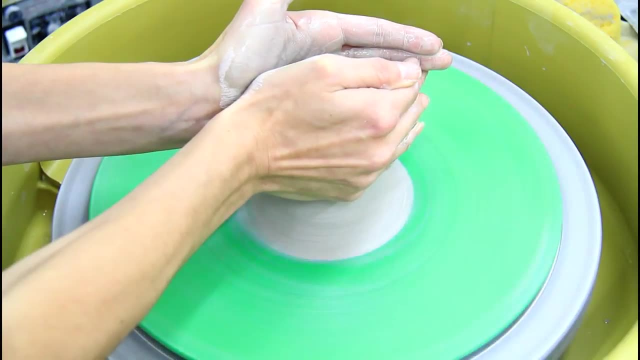 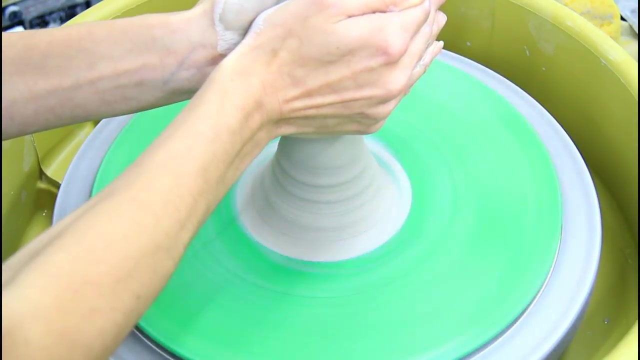 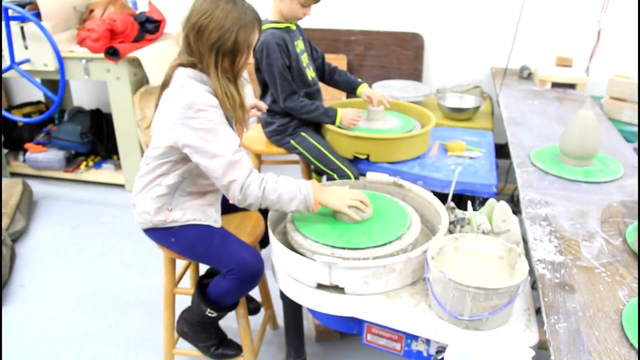 it too far this way And then I just lift, just ever so slightly going up. You see why it's called a cone, and this takes a lot of practice. So today we're going to just practice making cones, because that's the first thing that you need to know how to do. 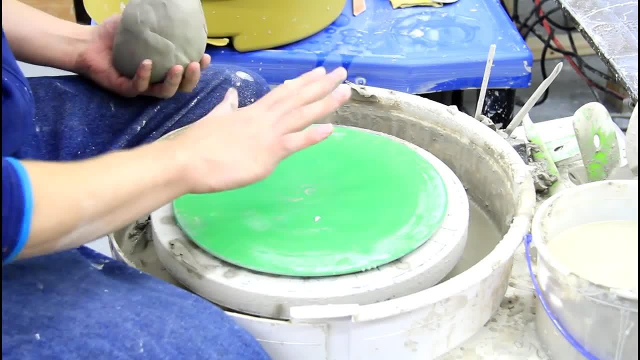 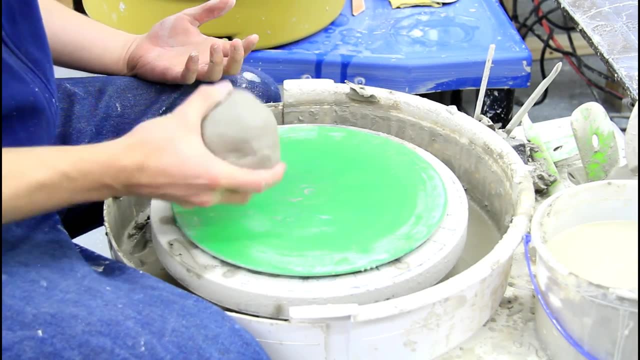 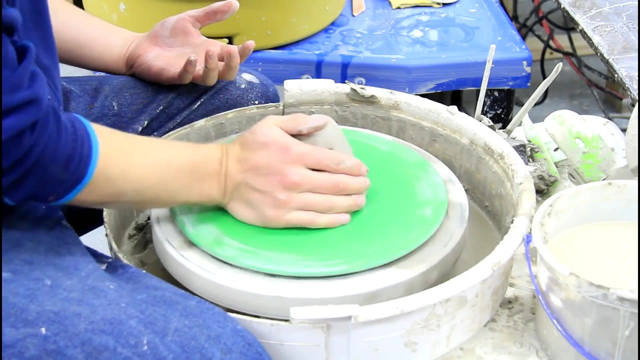 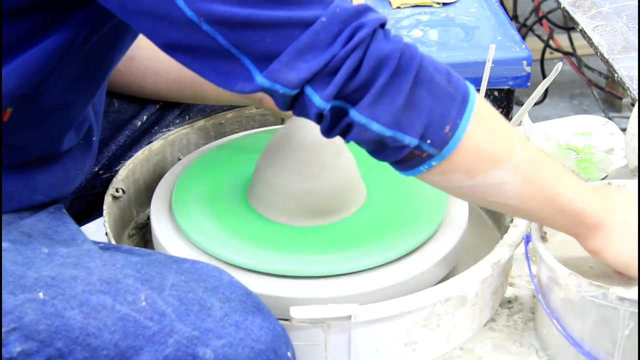 Thank you, Matthew at Valley Pottery, for demonstrating how to make pottery for us. And this looks like about two and a half three pounds of clay. Is she gonna make the tear things? Sure, I can make one of those tear drop things. I'll make a smaller one. So putting it down in the middle and then with some quick magic touches. 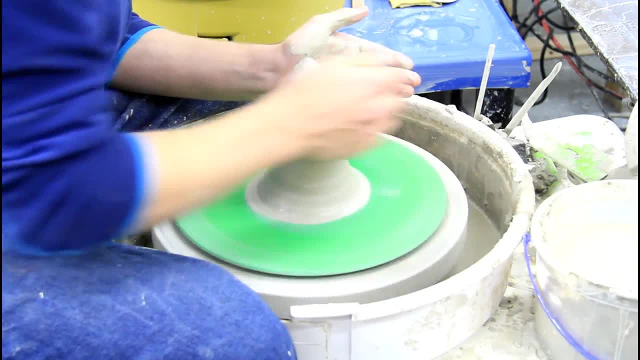 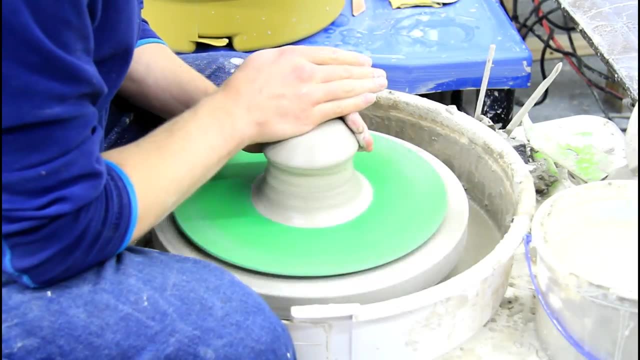 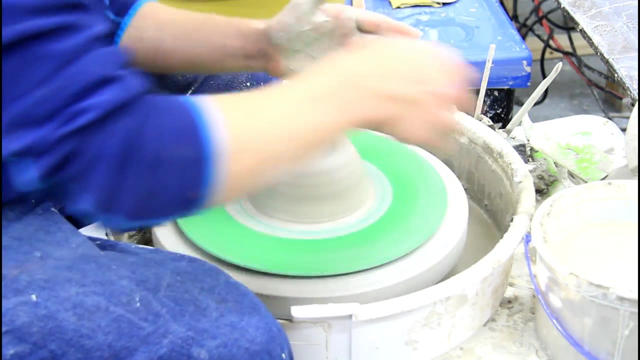 coning it up And then coming back down and centering the clay, so that all the centering is just having the two hands work together to kind of give the piece a massage on the shoulder- which is a tongue twister for me, unfortunately- So you know, just kind of moving it so that the clay gets more and more. 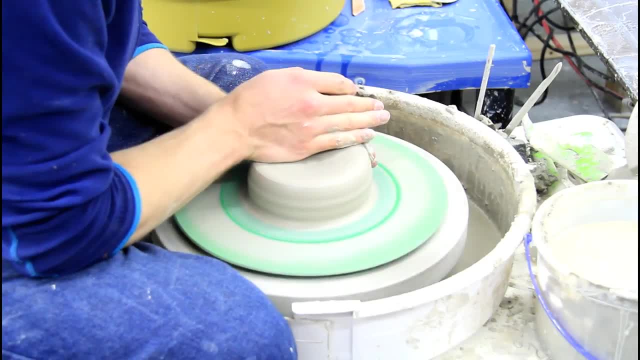 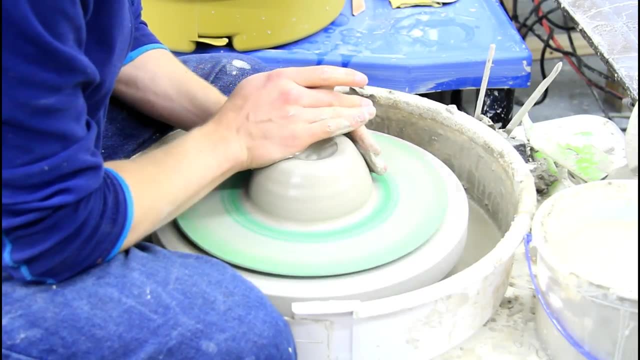 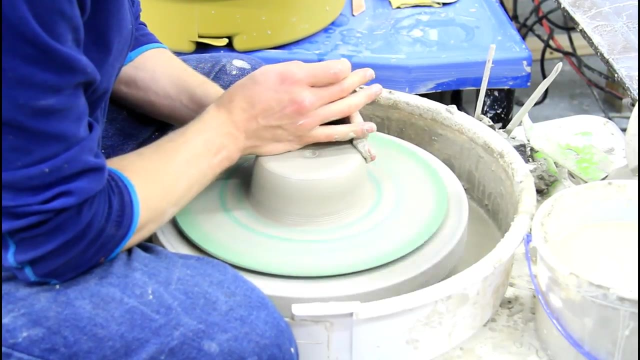 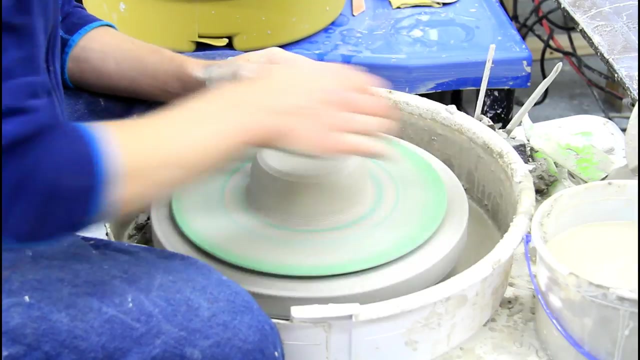 centered by moving the clay but holding it still at the same time, And there's a lot of quietness, Finesse and the hands working together to get the clay centered. After we're done with that, come in and open up the clay, And this from centering everything happened. 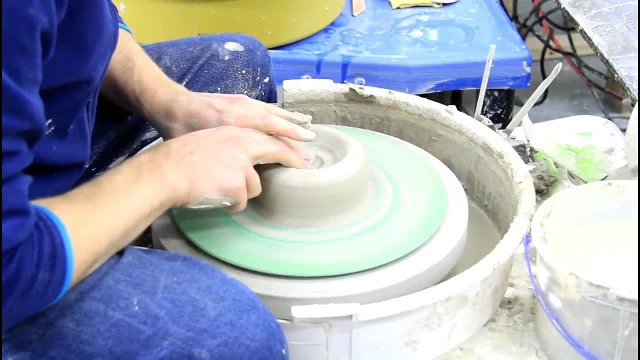 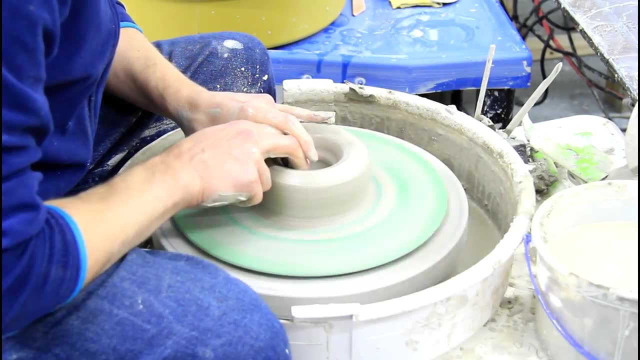 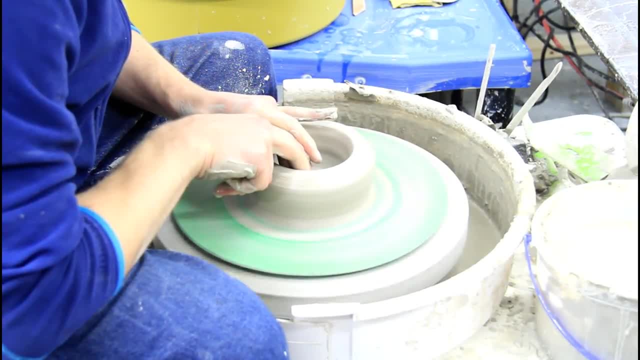 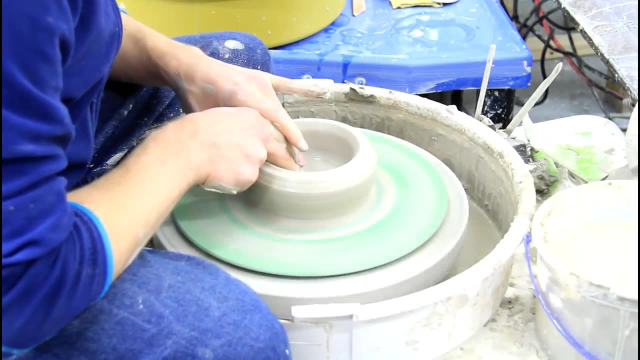 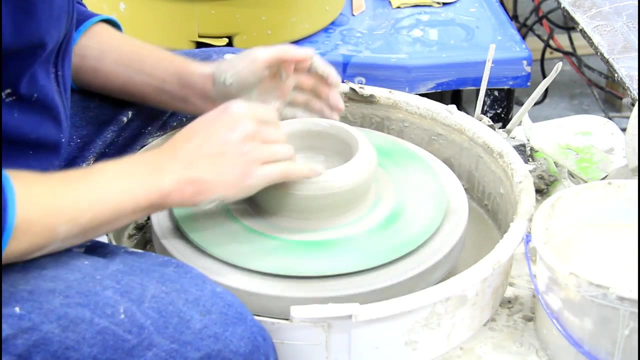 tear drops, which has more of a rounded bottom, so I end up opening it a little bit differently. so it's a rounded opening. Ah, it's still coming back. Nice smooth metal. And then we get to some of this cheating stuff of pulling everything back in. 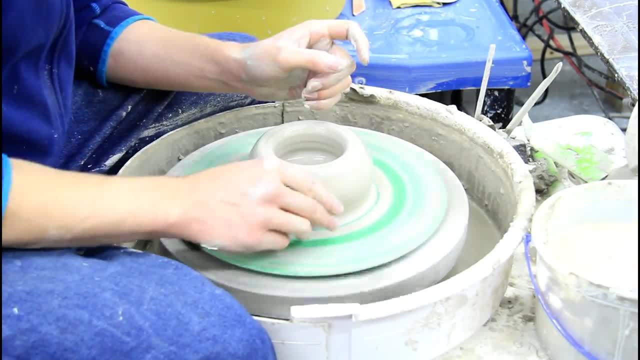 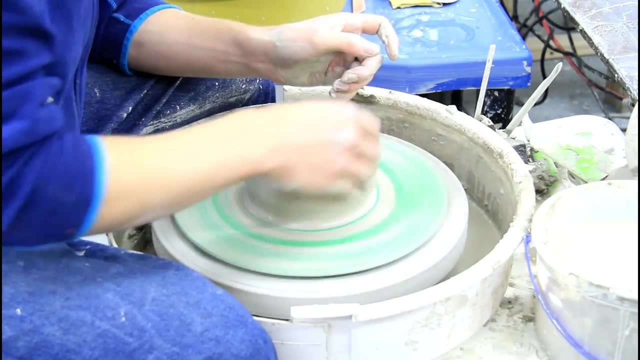 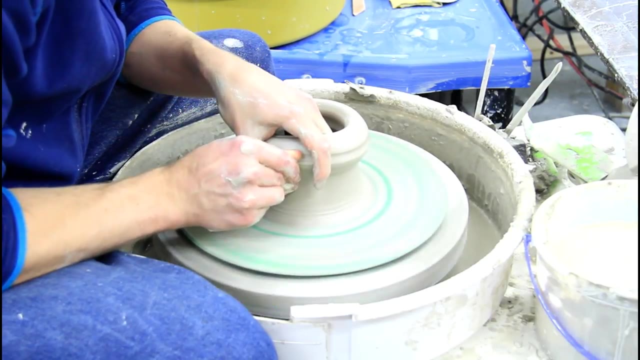 And then the real magical step of pulling. And what I'm trying to do is get my outside hand kind of hooked underneath so I can lift and pull the clay up. And I actually kind of like to call it lifting the clay, Slowing the wheel down and getting the clay moving upward Gently up. 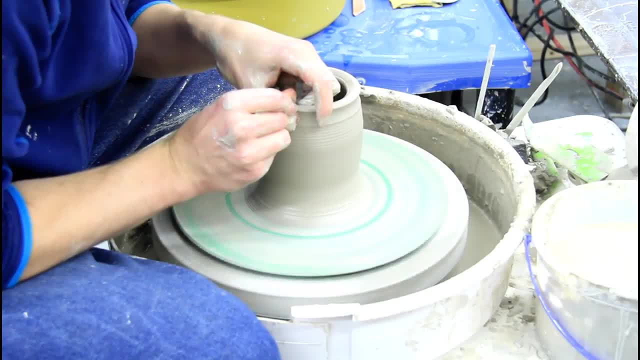 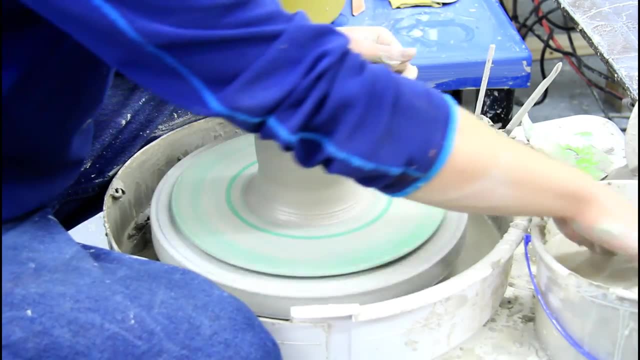 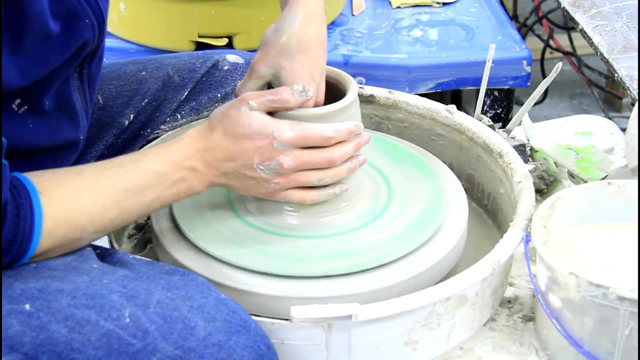 And most of the work, most of my focus is on the outside fingertip. Um, as I get to the top- kind of easing up Pressure- I have to keep everything really smooth so that my hands can flow past the clay. so I add in a little bit of water. 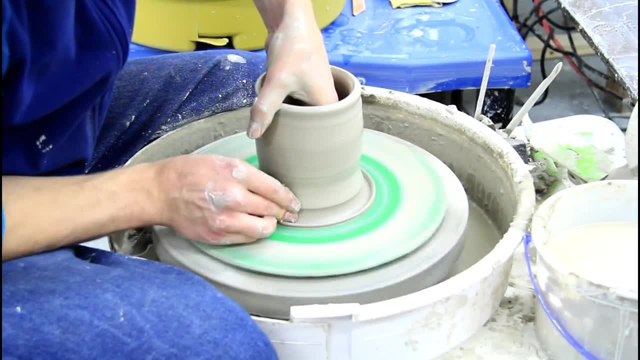 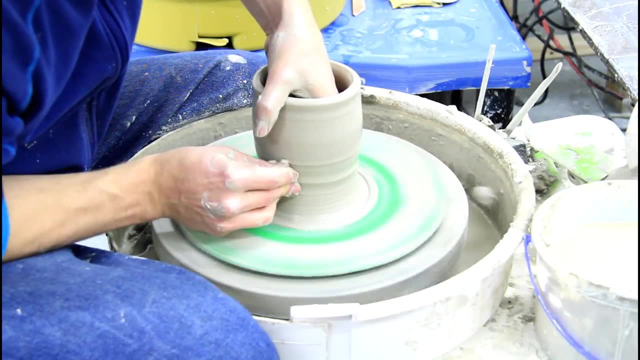 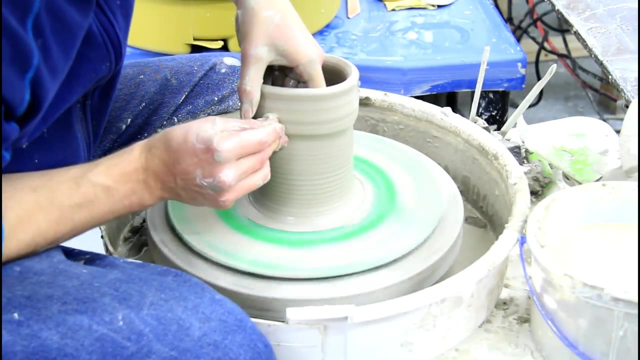 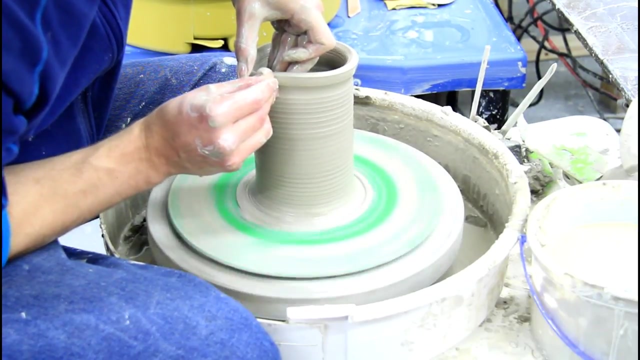 And then starting all the way bottom, creating a little bit of a notch so that I've got something to grab onto, And lifting that clay upward and inward. There's a real tendency for the clay to want to fly, So we have to kind of constantly work to keep it back inward. 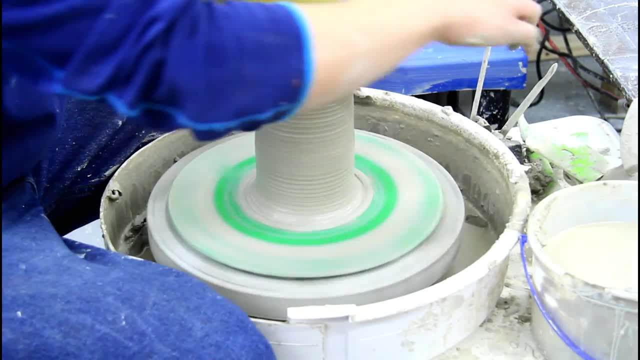 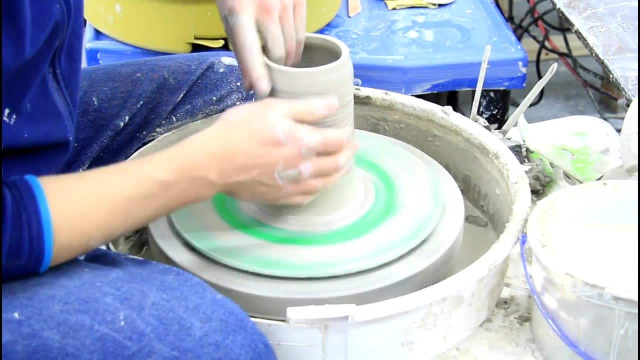 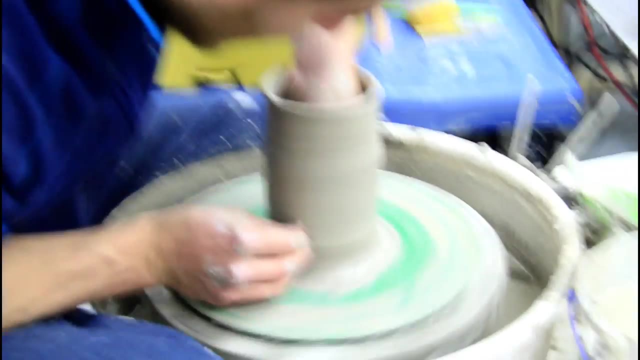 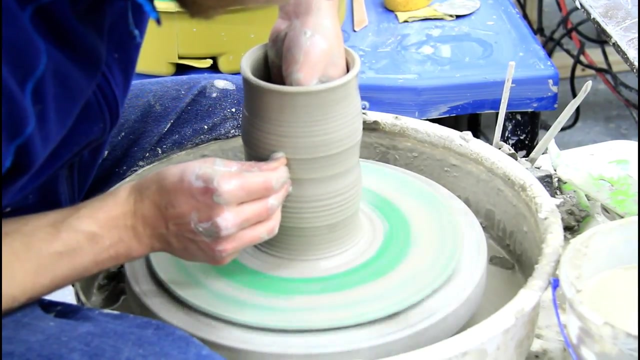 So normally I do three pulls. So that was the second pull. The dog's playing. I did all the crazy stuff with the dog So he stays. He's very careful And I do a lot of cheating So, like on this one, I'm actually doing a lot more of my lifting from the inside. 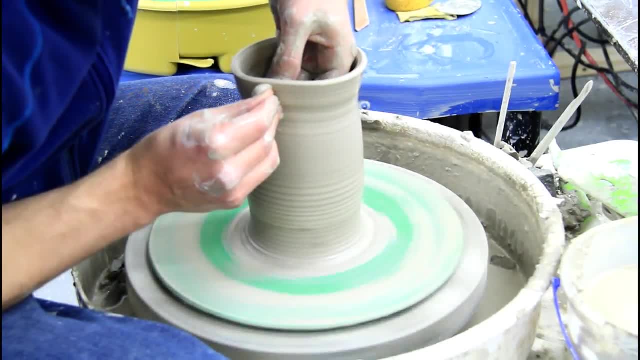 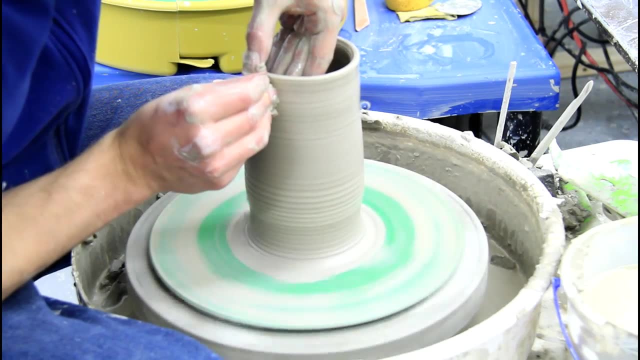 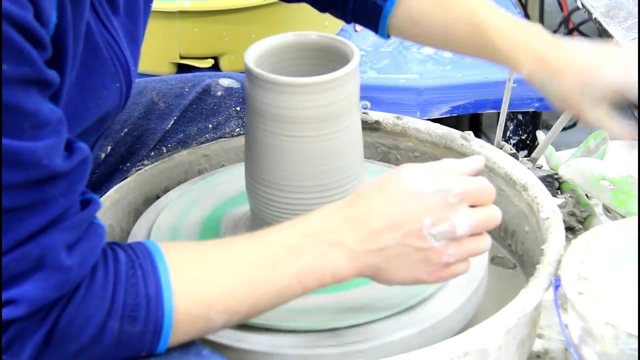 And the outside of my body Switches around. There usually isn't a right or wrong way to do any of these stuff, so After I'm done pulling, we pretty much have the final, The maximum height that we can get out of the piece. 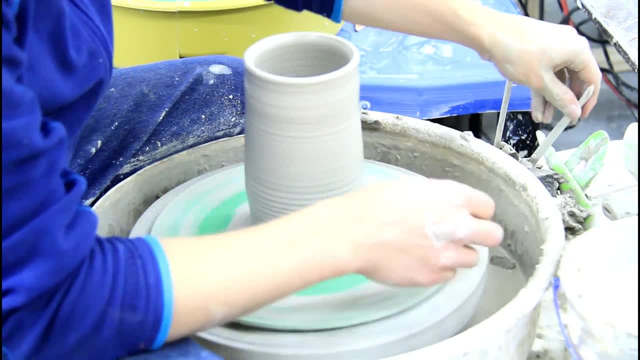 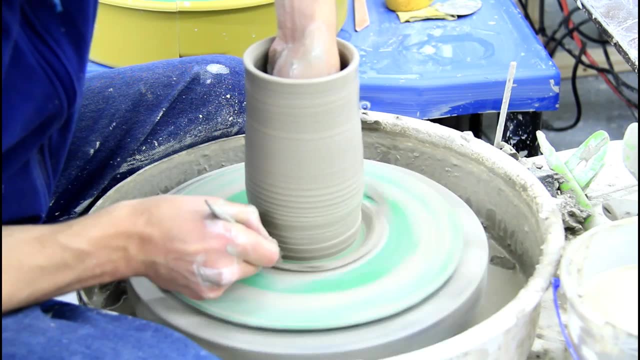 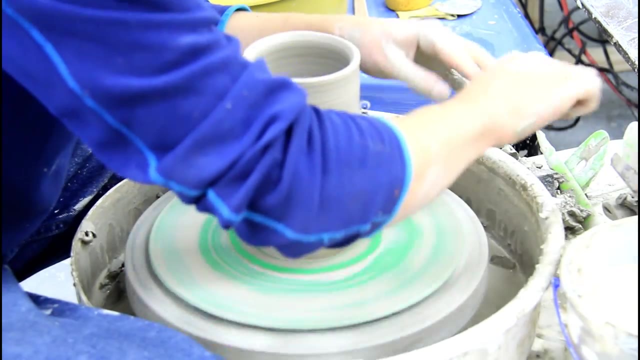 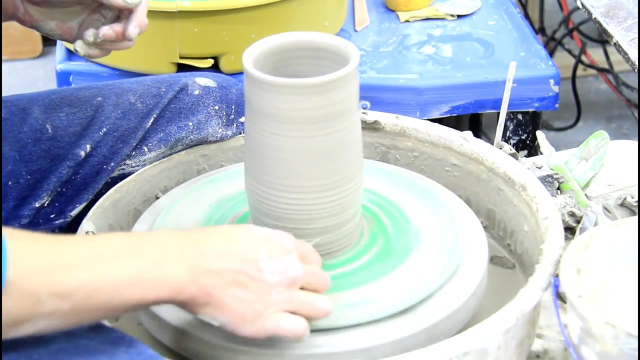 And then we'll start shaping it. First, take away some of this extra clay. Notice how he uses that tool. So that's the wooden knife, as they call it Just. And then, Because I'm OCD, I have to clean up Like that. 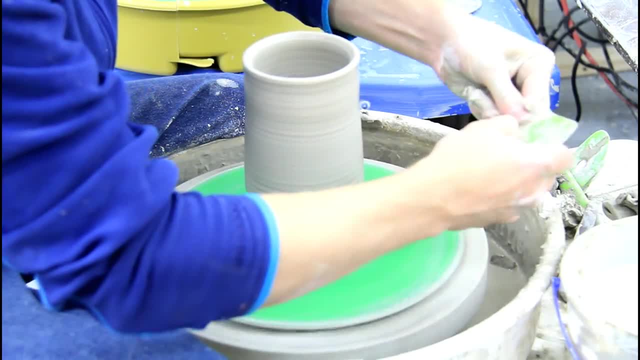 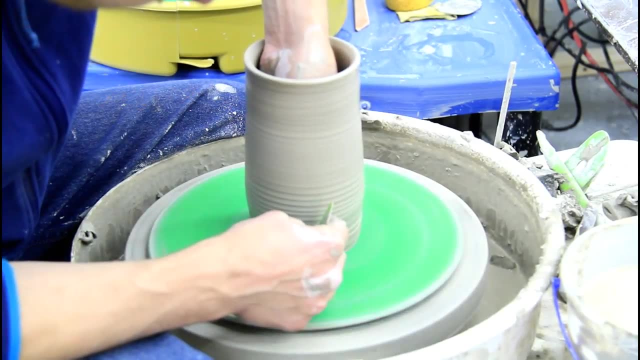 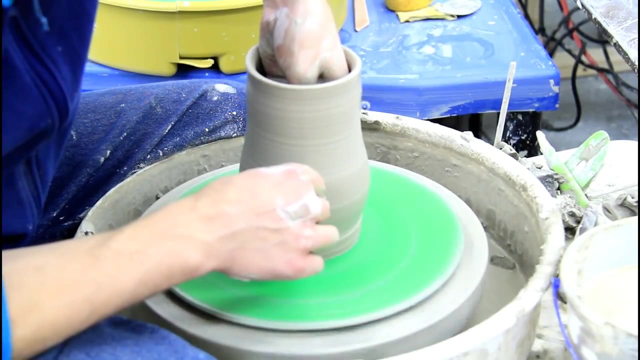 Makes it nice and bright again. And then I just like using this tool, This particular rib. So I'll start using a ribbon instead of my fingers to smooth things out, And I'm gently pressing with the inside hand And controlling it out with the outside hand. 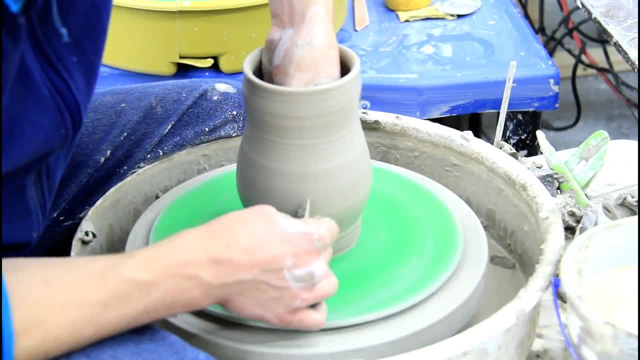 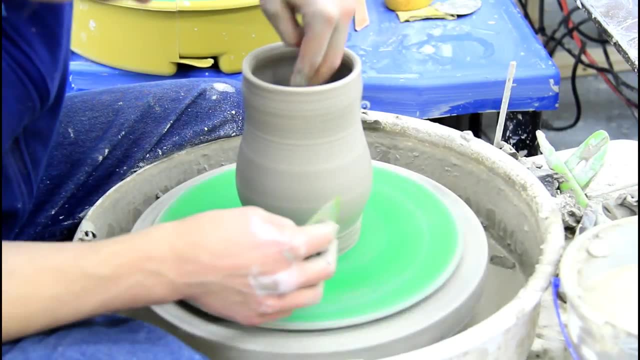 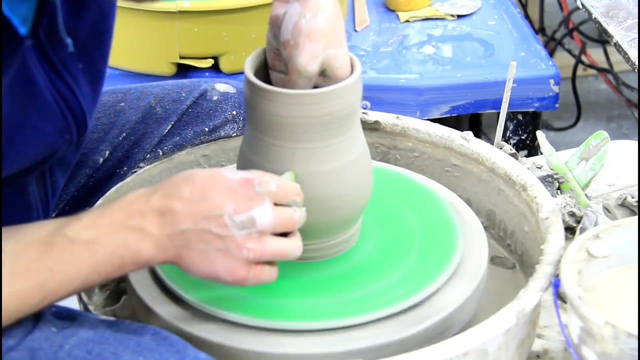 To create my shape. These pieces do get trimmed, So After a day or two of letting them sit, They It turned upside down and They cut away the extra clay from them. so Right now on the wheel, I'm not going to worry about. 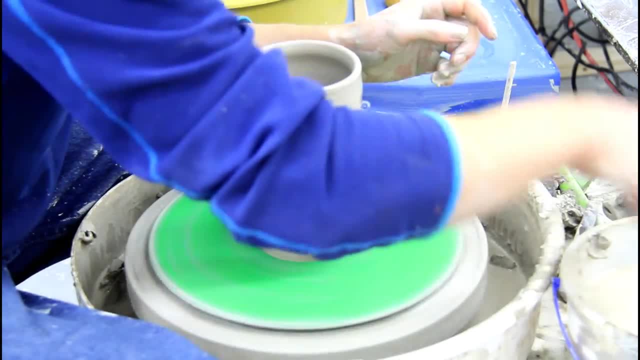 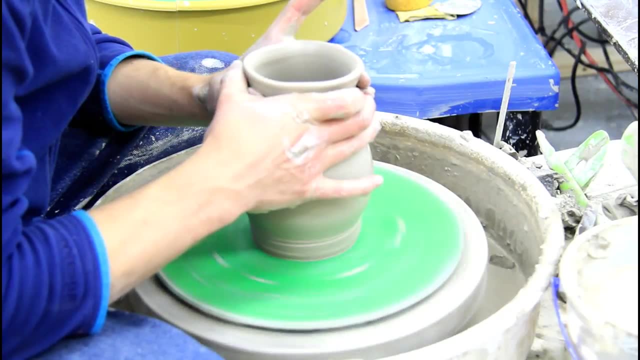 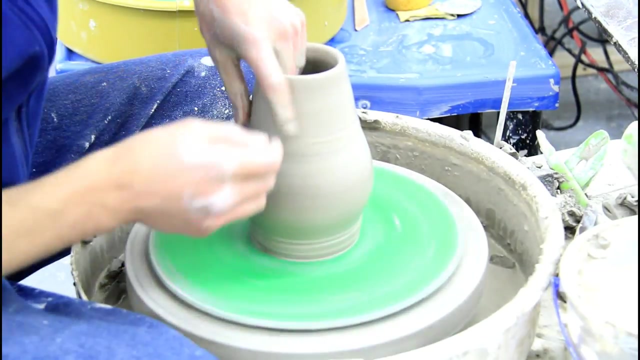 That ragged bottom Because it will get cleaned up. To actually make this cone, I have to collar the piece in, Just kind of like making a bottle, And then just collar it in So that the clay gets a little bit thicker. 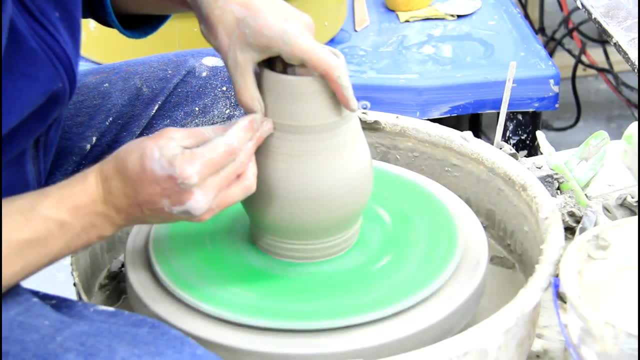 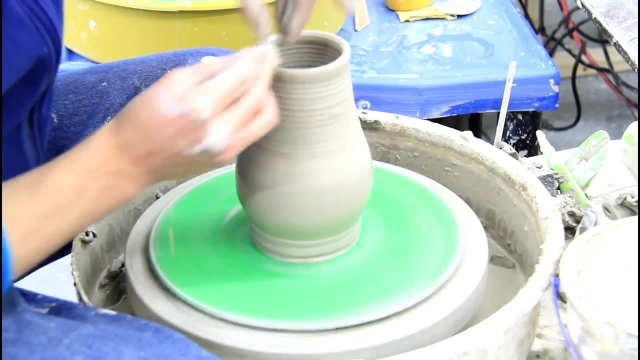 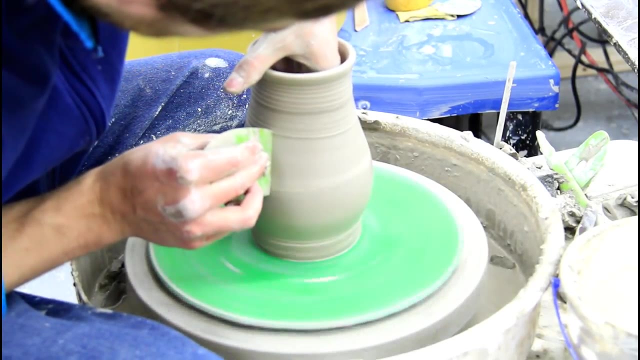 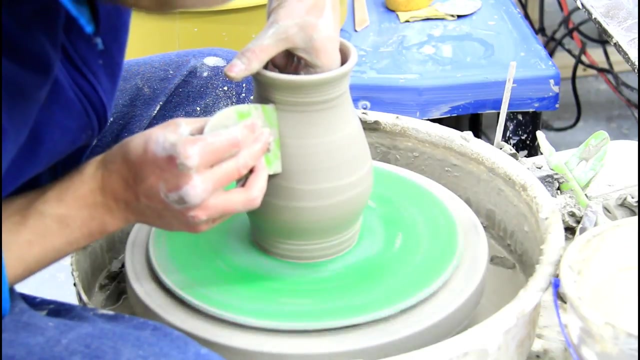 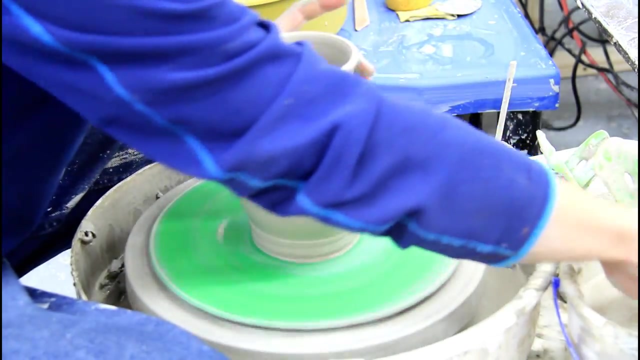 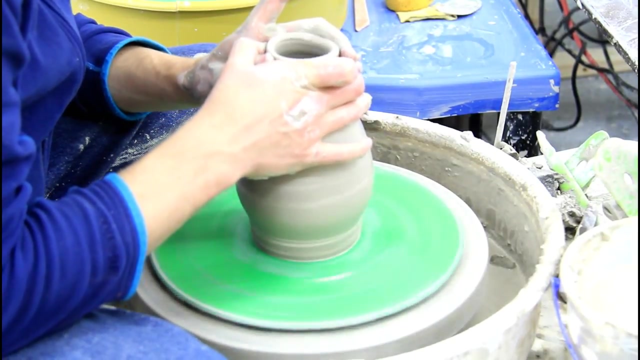 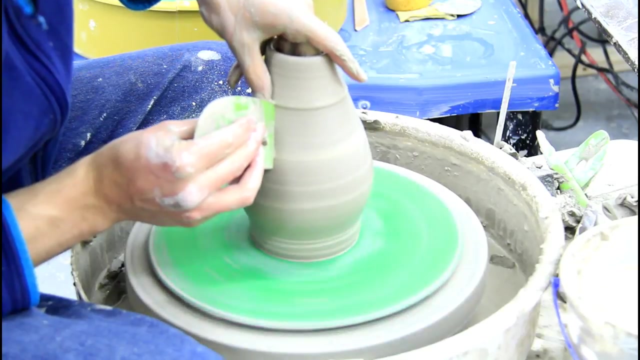 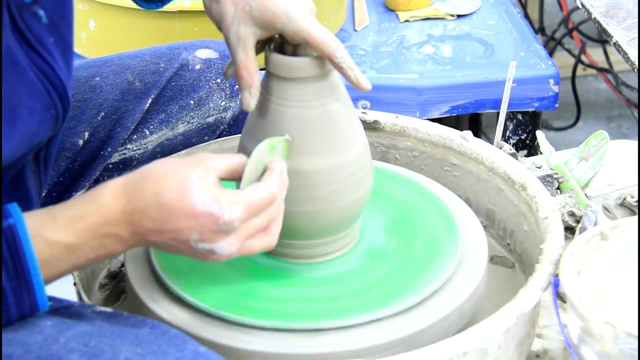 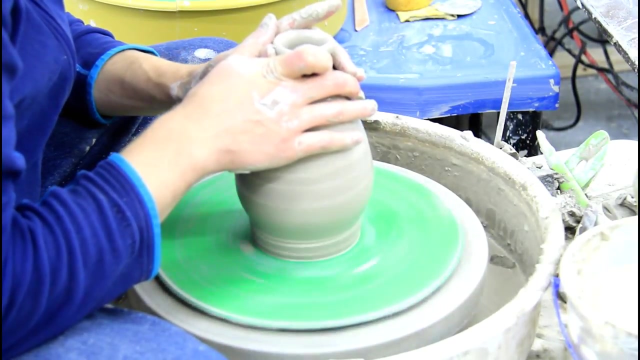 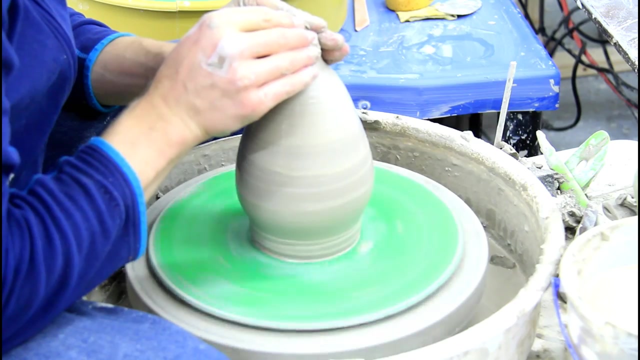 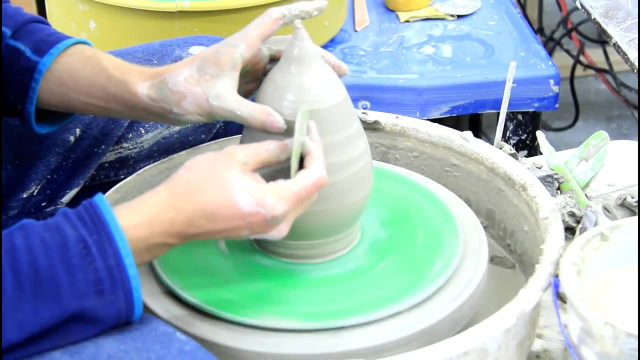 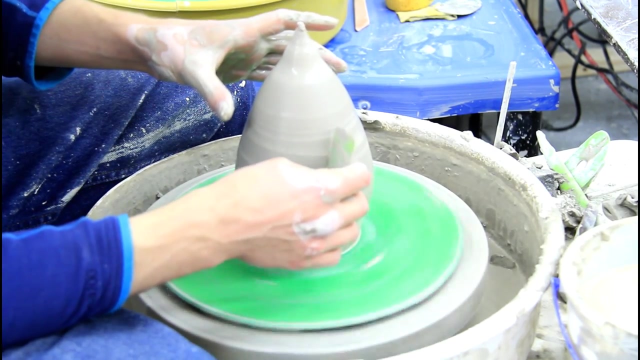 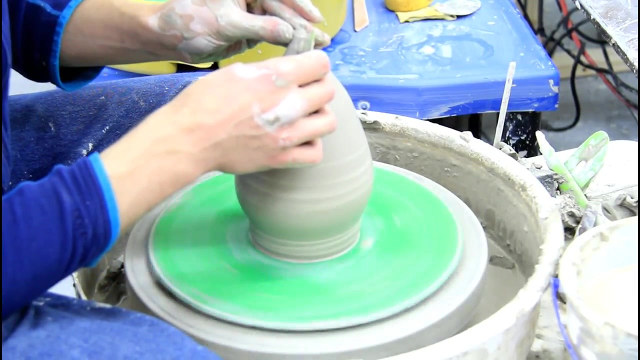 So I can come back and do another hole, Awesome, Collaring it in Super relaxing. I remember Finish that off, Pop it closed, Pop it And then Pass it in the glass And I actually leave the top Also, kind of. 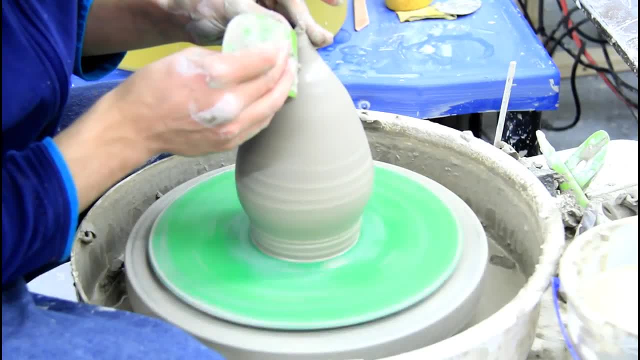 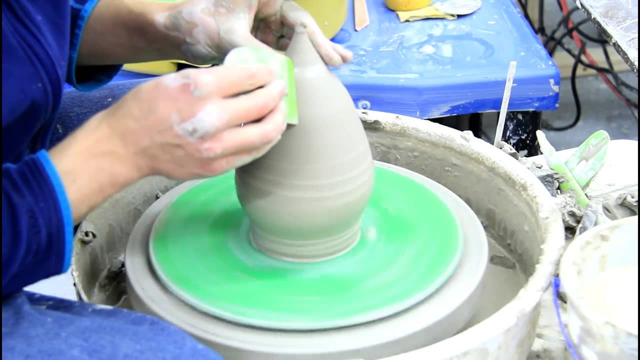